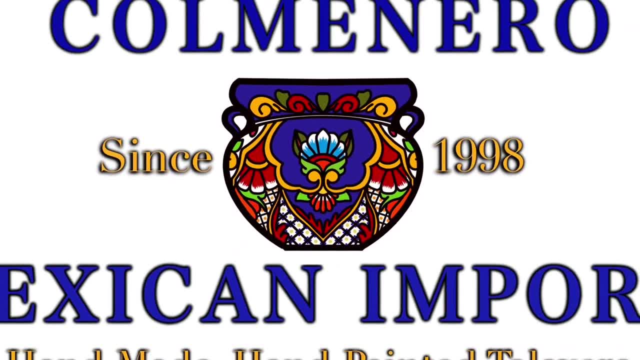 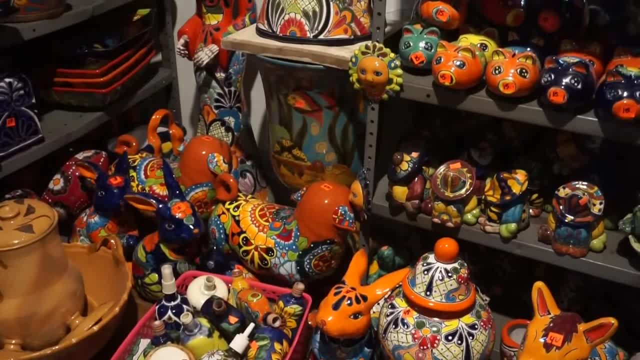 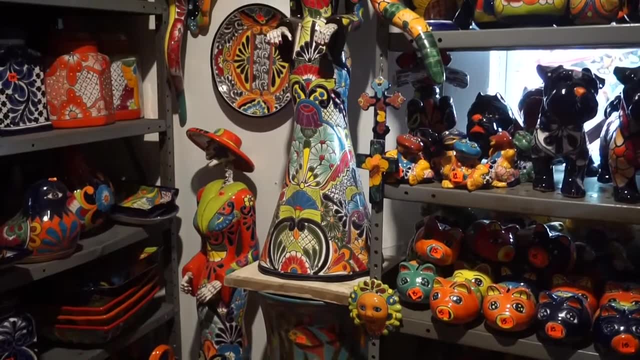 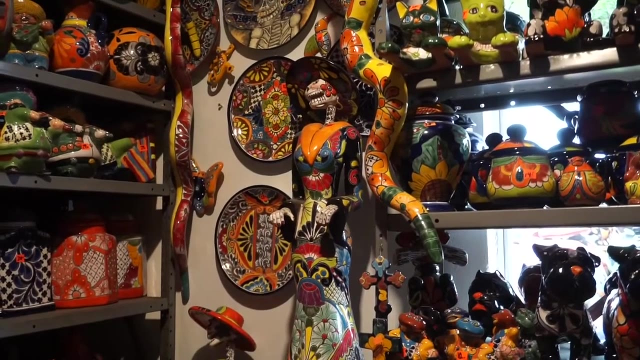 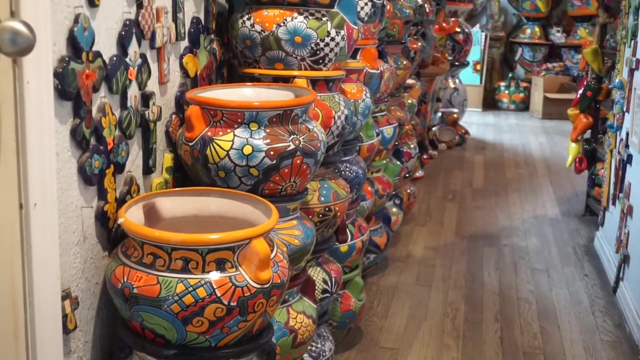 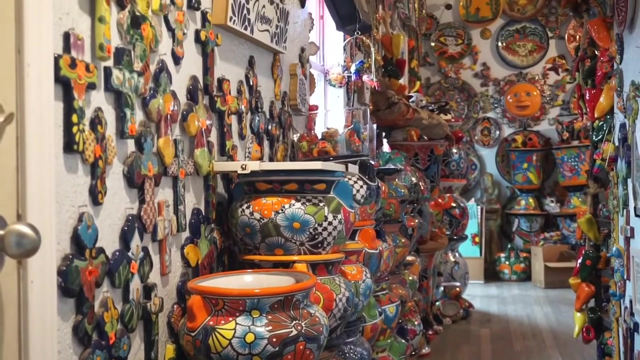 Talavera pottery is a type of Mexican ceramic art that features brightly colored designs and intricate patterns. These patterns often feature floral patterns and other traditional motifs. It originated in the city of Puebla and is known for its use of cobalt, blue, yellow, green and black glazes. 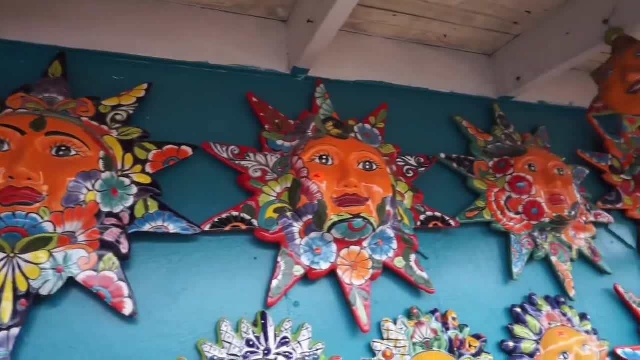 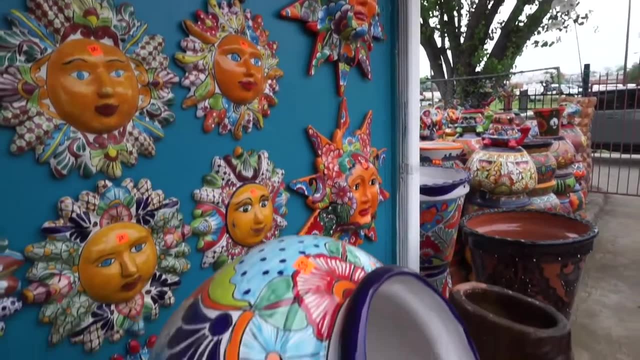 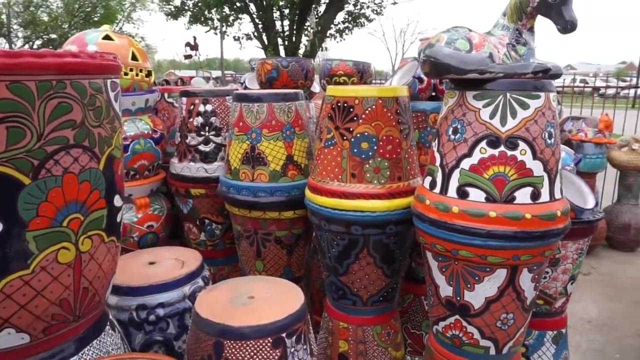 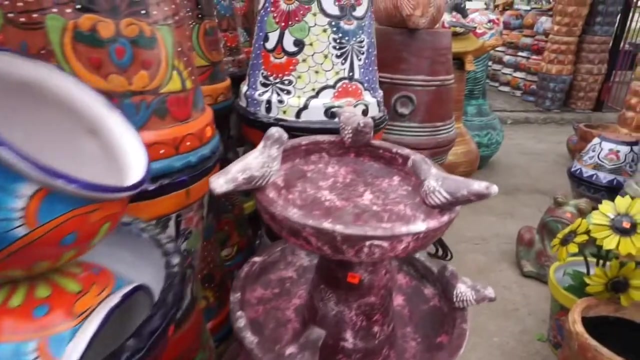 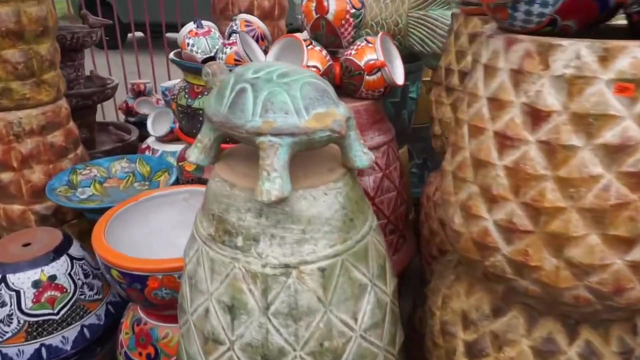 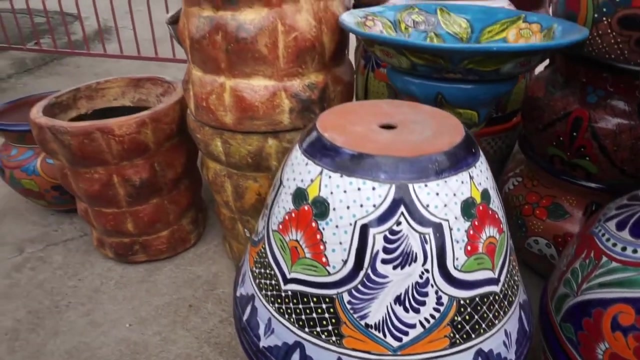 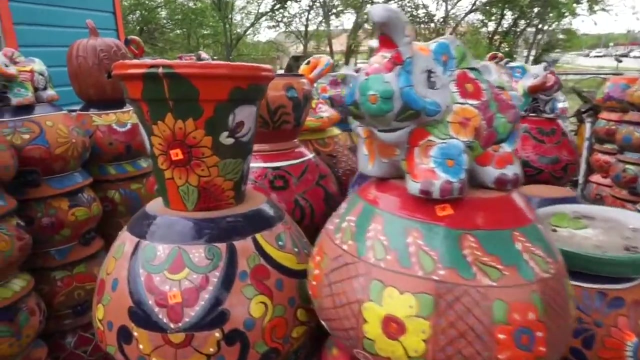 Talavera pottery is traditionally handcrafted using a combination of indigenous and Spanish techniques, including the use of a potter's wheel and hand painting with natural pigments. Some of the most common designs found on Talavera pottery include floral patterns, geometric shapes and animals. These designs are often arranged in a symmetrical and repetitive. 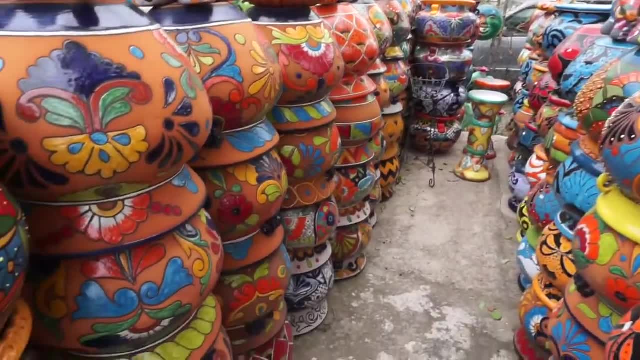 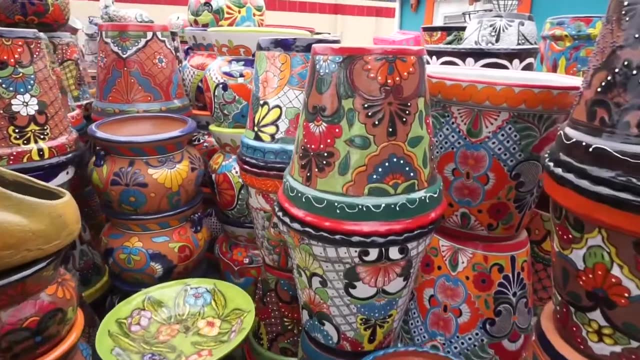 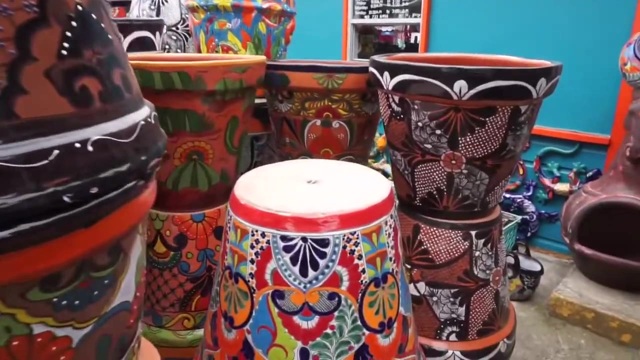 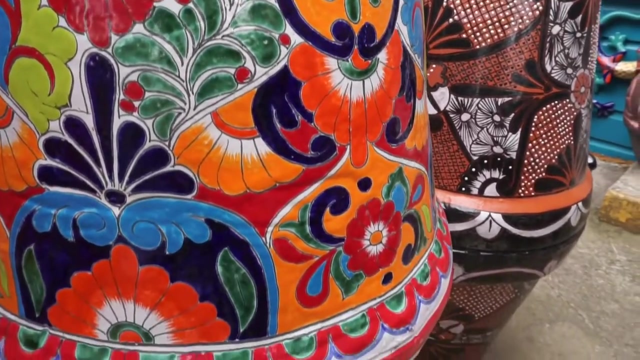 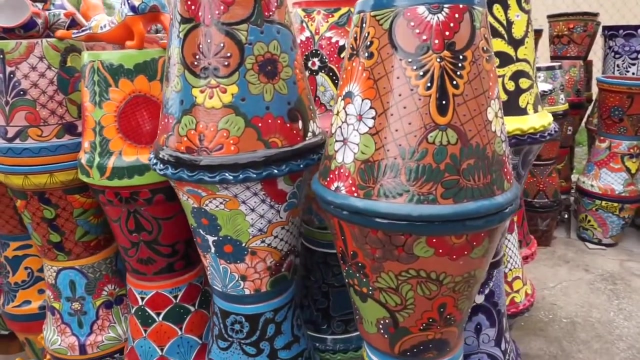 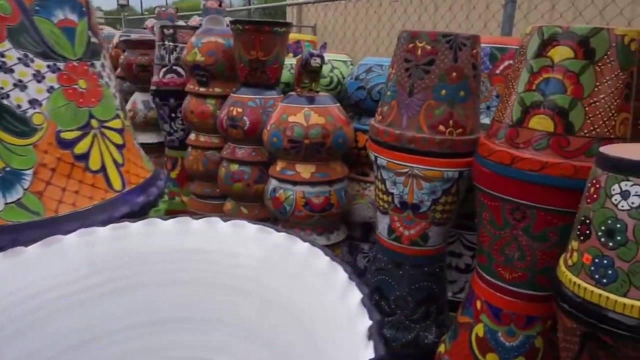 fashion, creating a visually striking and balanced composition. The floral patterns, for instance, may feature roses, sunflowers or other local flowers, while the geometric patterns are often arranged in lines, squares or triangles. The pottery is made using a unique blend of local clay and is 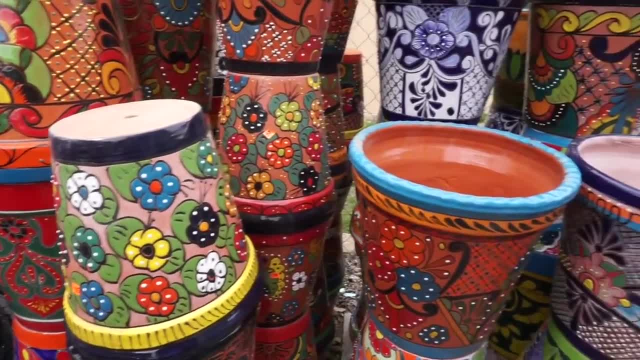 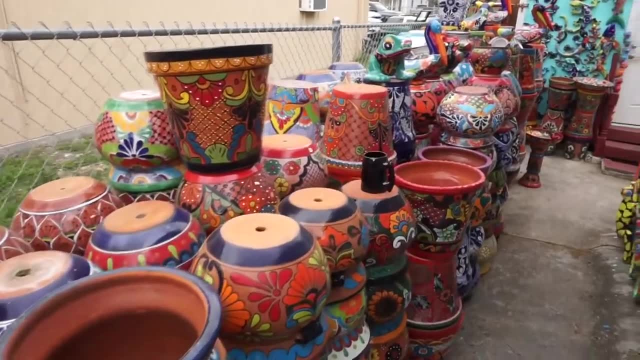 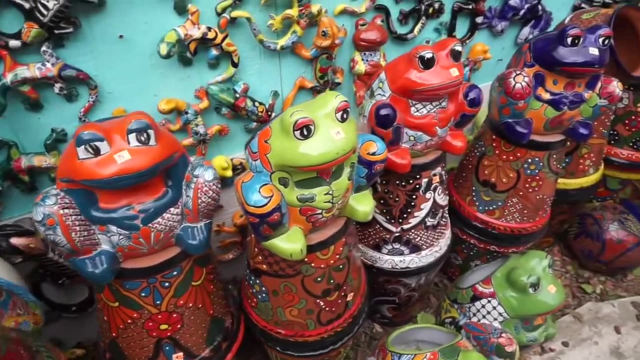 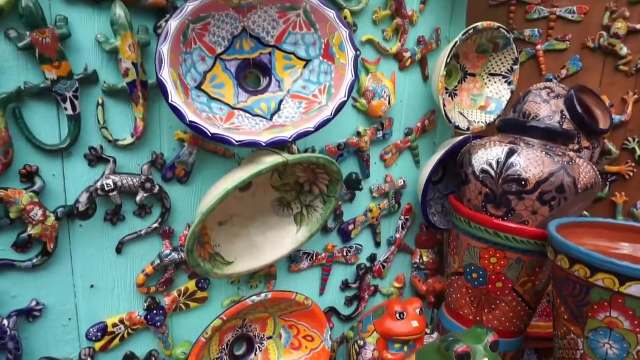 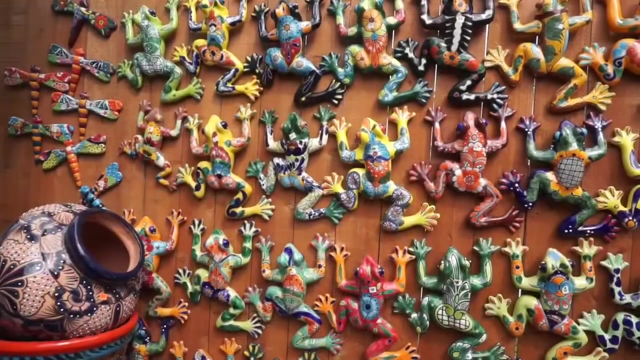 made using a unique blend of local clay. and is made using a unique blend of local clay and is hand-painted by skilled artisans using a combination of techniques such as underglaze, overglaze and barrobronido. The pottery is made using a unique blend of local clay and is made using a combination of. 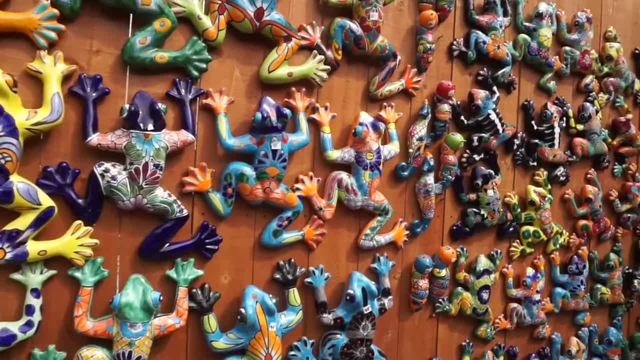 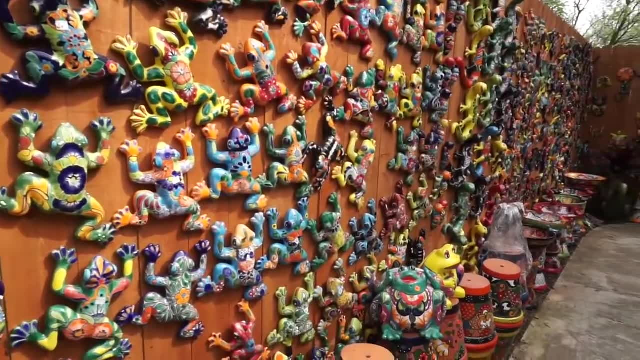 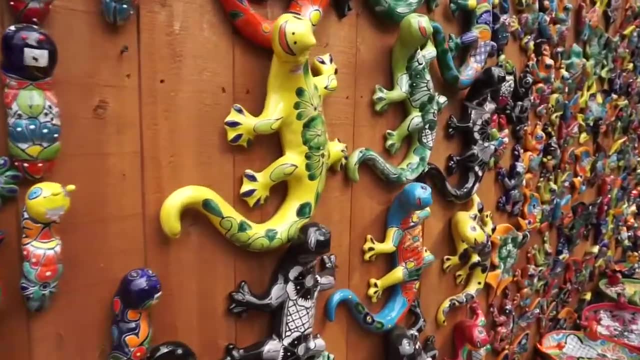 different techniques, such as underglaze, overglaze and barrobronido. Talavera pottery has become a popular decorative art form and is often used to create dishes, vases, tiles and other decorative objects. We import the pottery from Dolores, Hidalgo, Guanajuato, Mexico. Here the craft has been used to create a few of the most popular decorative objects. 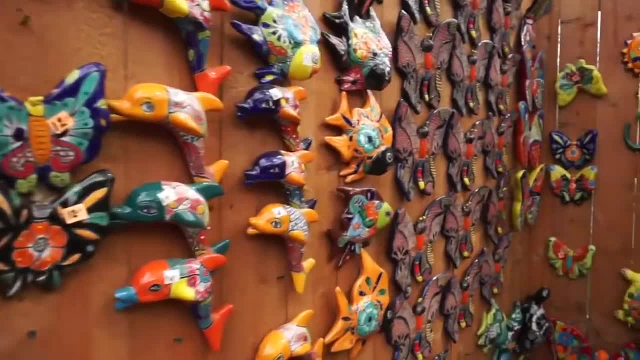 We import the pottery from Dolores Hidalgo, Guanajuato, Mexico. Here the craft has been used to create a few of the most popular decorative objects. We import the pottery from Dolores Hidalgo, Guanajuato, Mexico. Here the craft has been used to create a few of the most popular decorative objects. 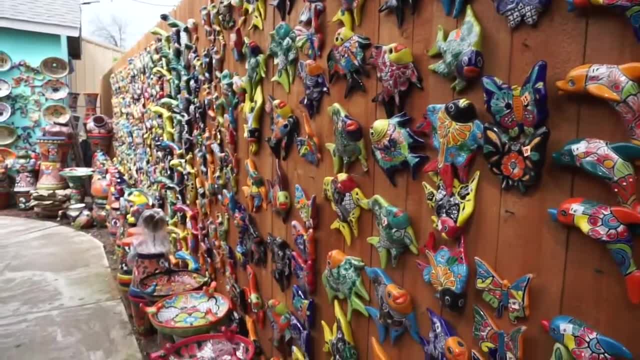 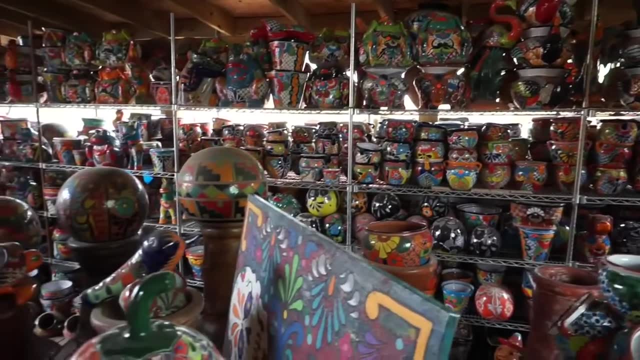 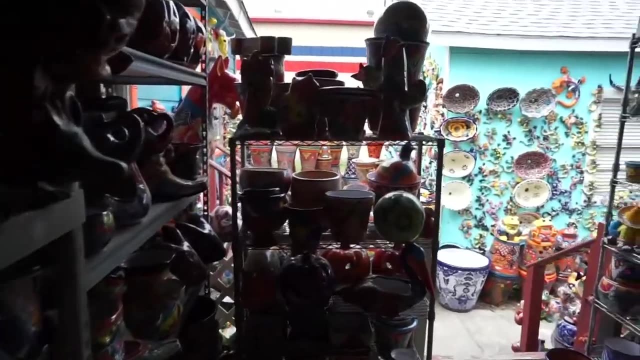 The unique style and quality of talavera pottery from this region has gained international recognition and has become a symbol of Mexican artistry and craftsmanship. In addition to its cultural significance, Talavera pottery from Dolores Hidalgo, Guanajuato, has played an important part in the region's economy. 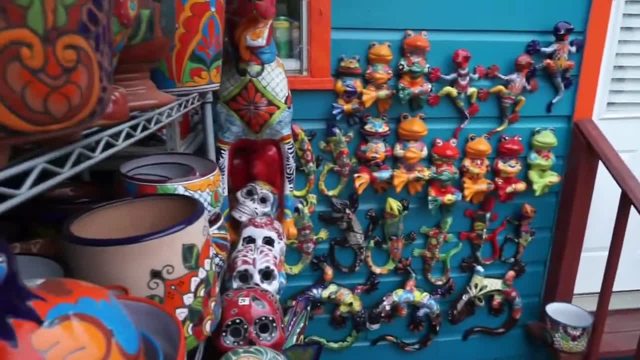 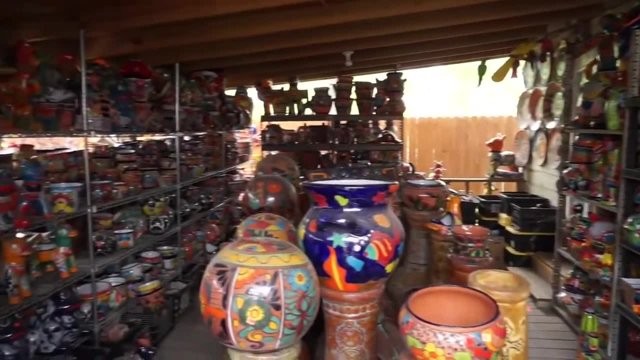 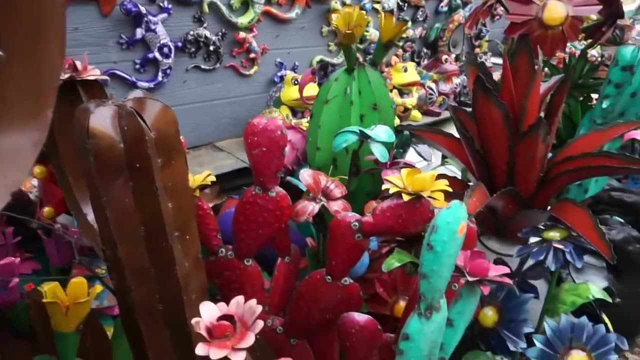 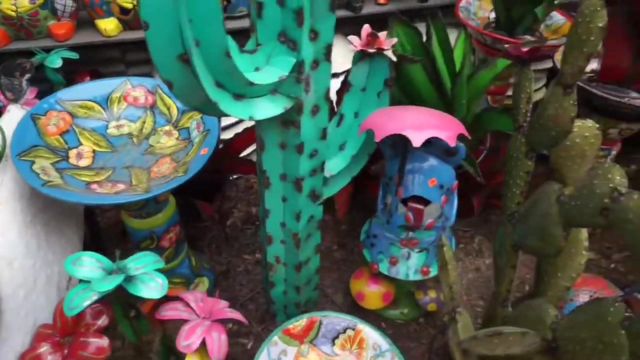 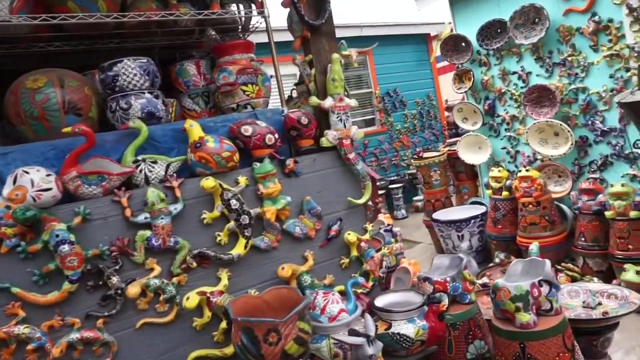 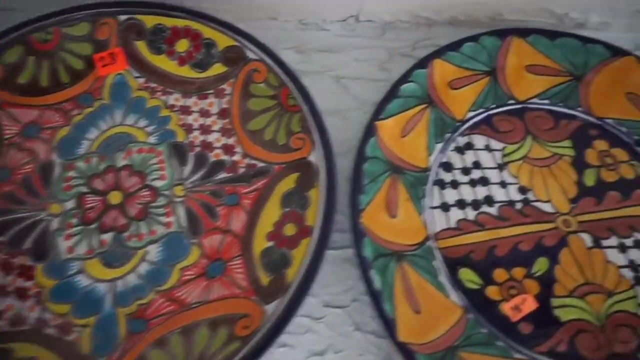 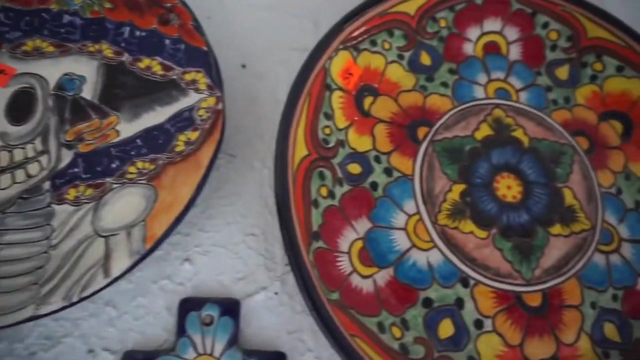 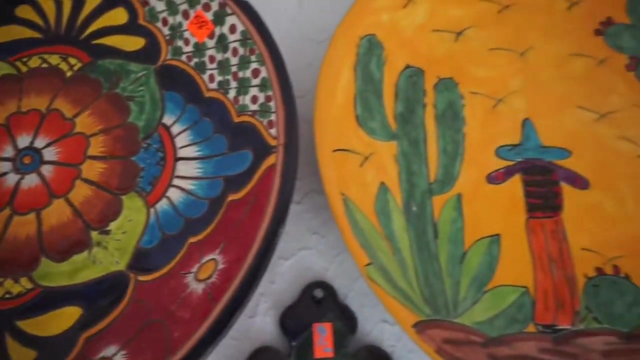 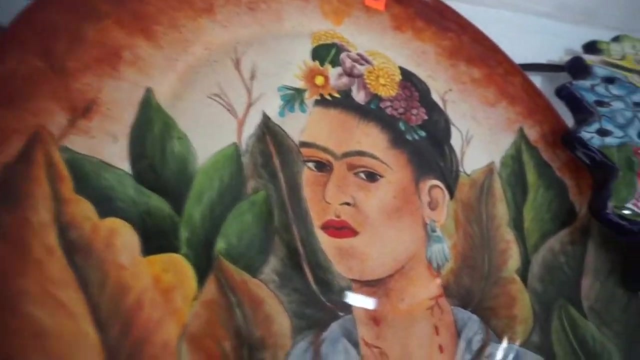 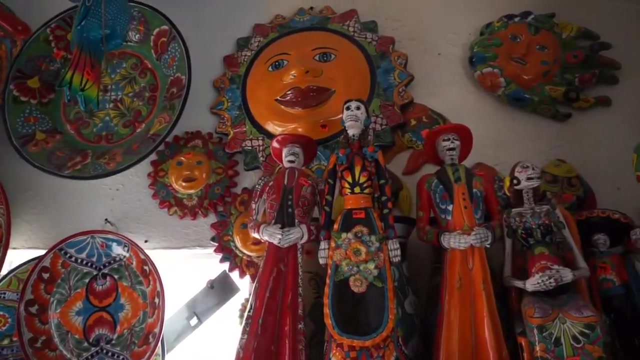 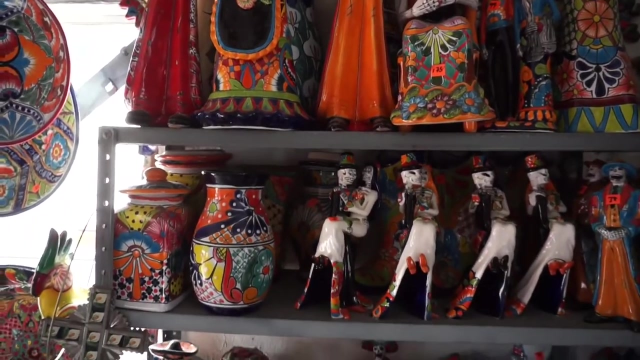 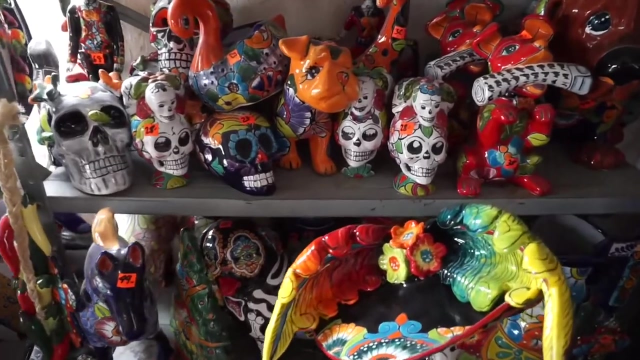 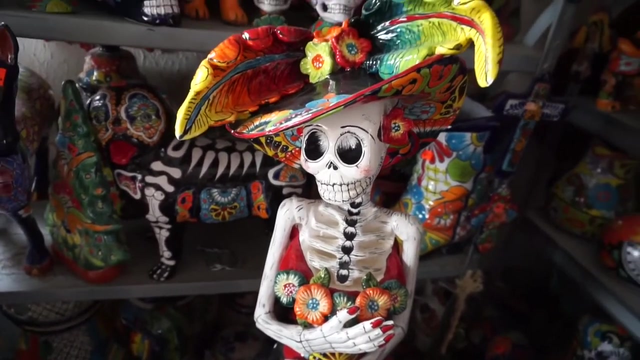 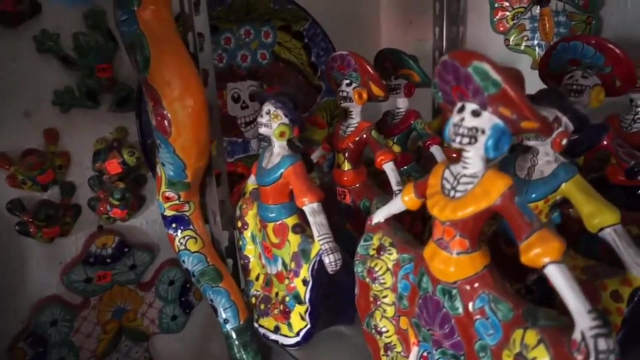 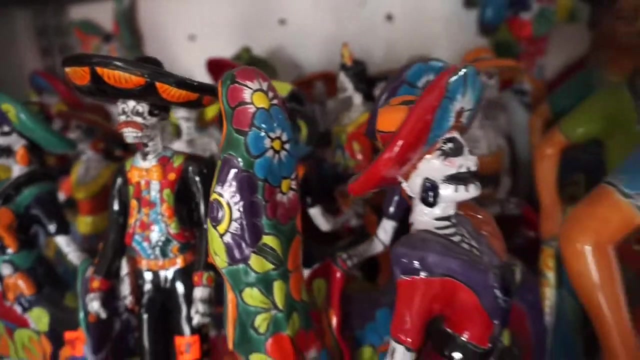 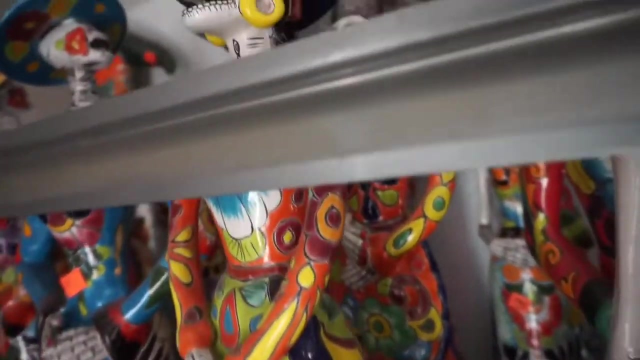 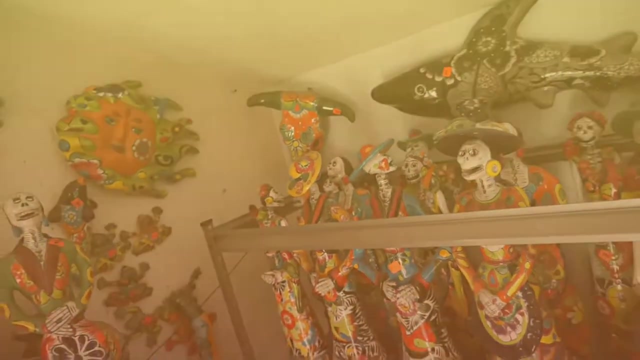 piano plays softly. Talavera is a unique art form that is a symbol of Mexican culture and history, and it is a cherished possession for many people. piano plays softly. piano plays softly. piano plays softly.